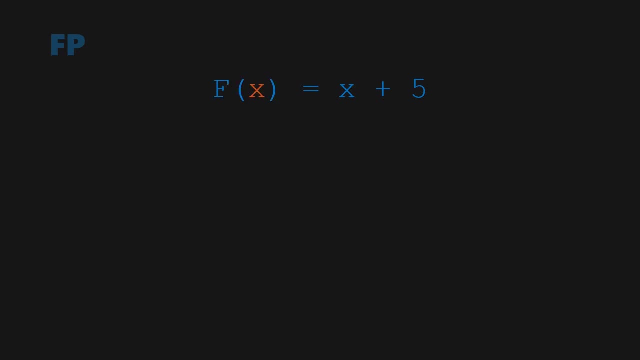 or even high-level calculus. The function f of x takes in x as an input parameter and returns x plus 5.. f of 10 returns 15,, f of 20 returns 25, and so on. If desired, these functions could have. 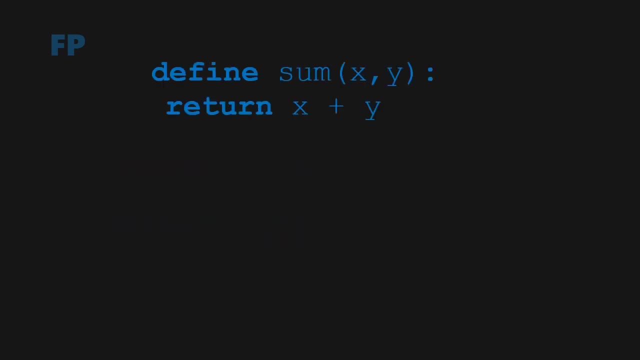 multiple parameters. The function sum, which takes in x plus y, takes in the two parameters and just returns their sum. Sum of 30 and 50 returns 80, and so on. This same concept of functions is widely used in programming, except its abilities and scope are heavily expanded. 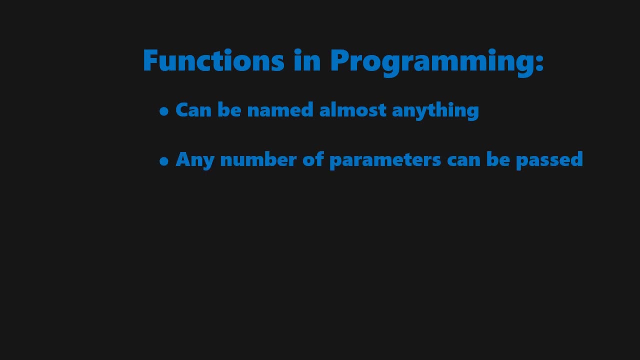 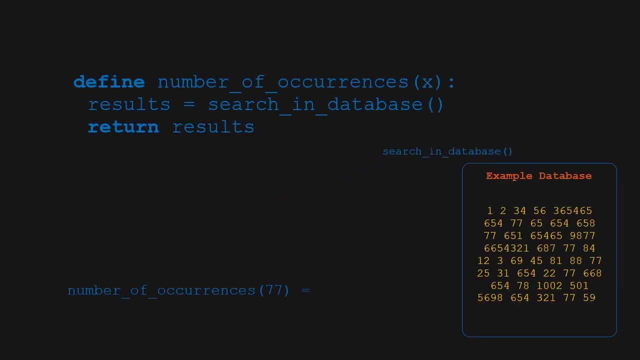 Functions can be named almost anything and an infinite amount of parameters can be passed into them. They can also return anything imaginable. For example, functions can be made to accept a number as a parameter and then take that number and search for it within a database. 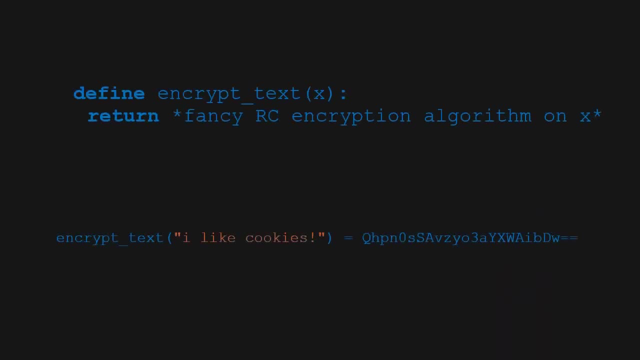 and return the result. We could also have a function that takes in a piece of text as a parameter and returns it encrypted. But let's get back to functional programming. A number of requirements need to be met when programming in this way. These requirements are almost all. 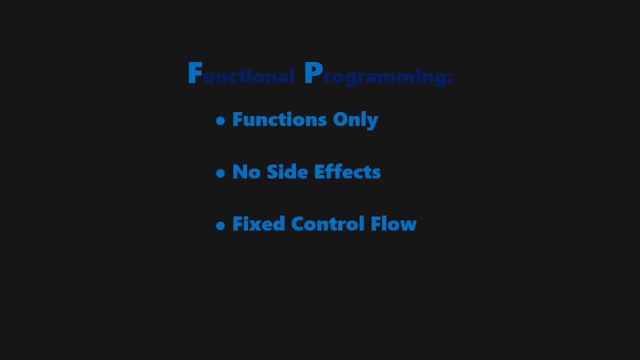 functions, only no side effects and a completely fixed control flow. To explain some of these parameters, let's look at a simple problem. Let's say we want to write a function that takes two numbers and just returns their sum squared. We'll take two approaches to this problem. 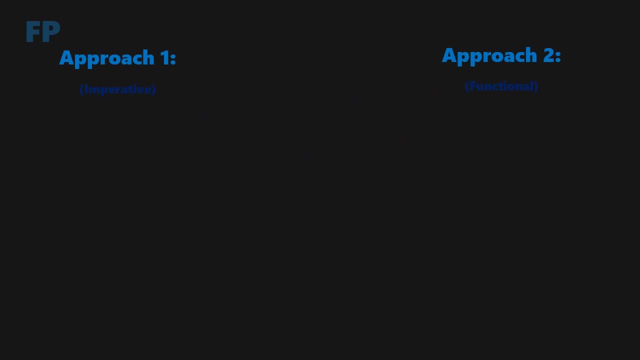 One functional and one less functional or imperative. Let's start by defining a function called squaredSum, which takes in two parameters: x and y. Within the function, we define a variable called sum, which stores the sum of x and y, Then define another variable called square. 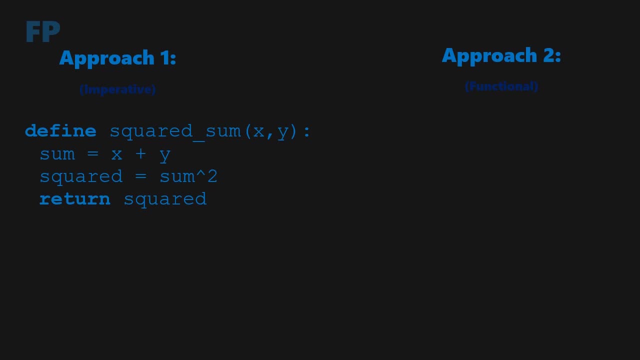 which holds the value of the sum raised to the second power. Finally, the function returns the variable squared. So if we were to pass two and three within the function squaredSum, the variable sum within the function would be five and the variable 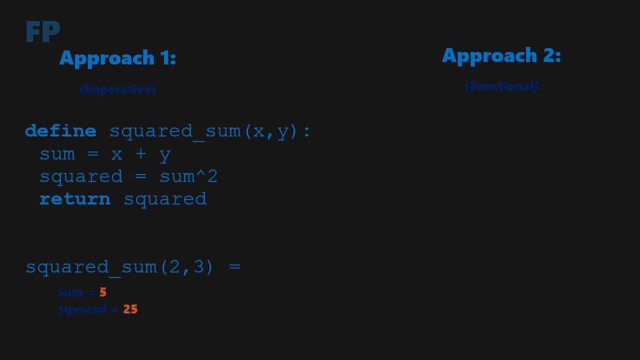 squared would be 25.. Finally, the function would just return 25.. So the value squaredSum two three would be equal to 25.. Let's rewrite squaredSum now down to a single line. All we do is return x plus y raised to the second power, without storing any variables. 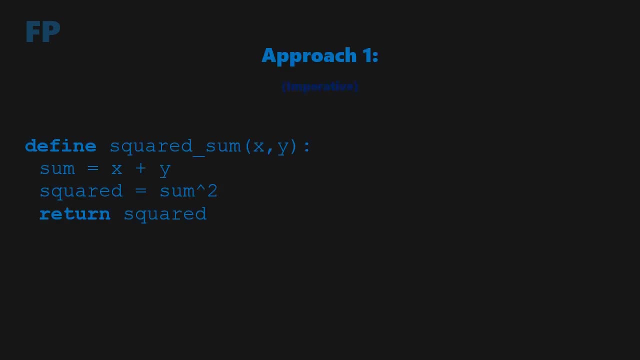 Can you see the difference between these two functions? In the first approach, we decided to store intermediate steps to the final solution within variables before returning the answer. The problem with using variables like this is the production of quote unquote side effects When looking at how a 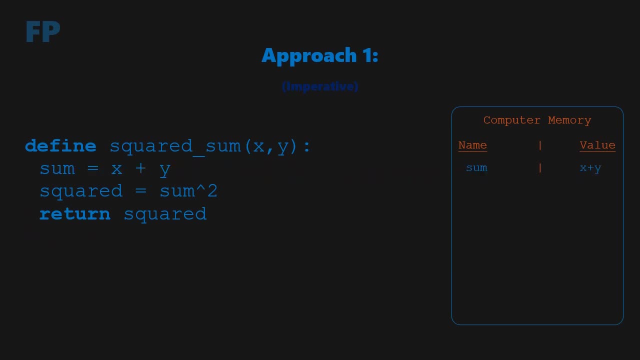 computer would solve the first version of squaredSum. the variables created, sum and square, have to be remembered by it and stored somewhere in the system's memory. This means that the function, when evaluating a given set of numbers, produces events outside of its own body and 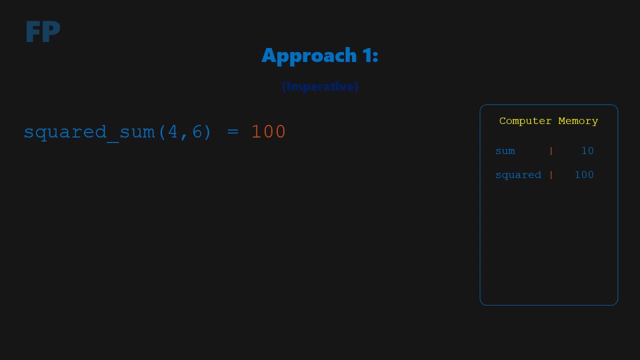 affects something else in another location, which in this case would be computer memory. These are called side effects, events that are caused by a system within a limited scope, whose effects are felt outside of that scope When systems grow and expand. the occurrence of side 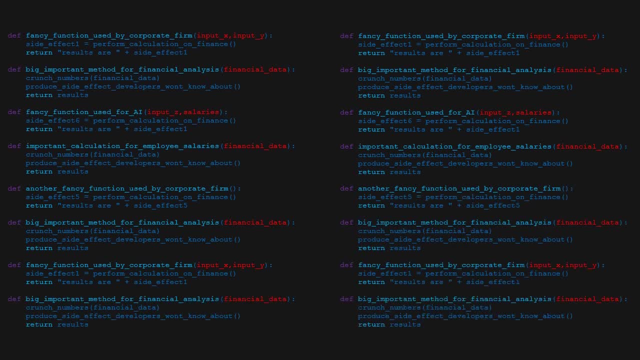 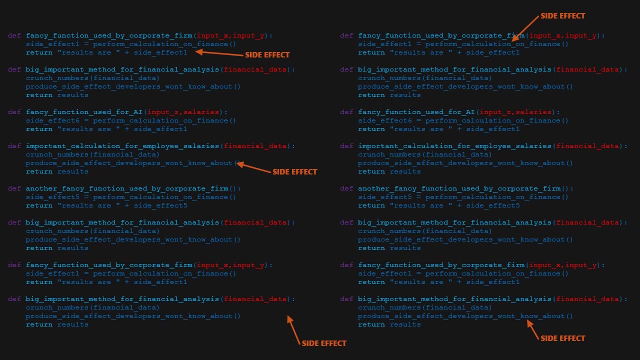 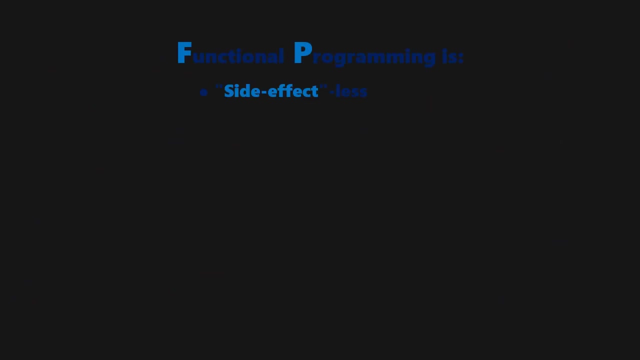 effects like these can be problematic. Due to the sheer scale and complexity some of these projects can get to, which would contain countless different functions producing side effects, it would become increasingly difficult to debug systems and find exactly the source of some given problem. This is one of the benefits of using functional programming: The side effects are eliminated. 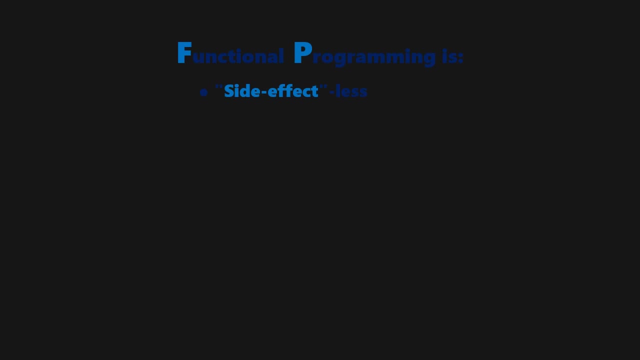 completely allowing for weird and unexpected bugs to be minimized and for developers to more easily understand the operations of a given system. Now let's look at the second version of squaredSum. In the function, no variables are used and the solution is directly returned without causing. 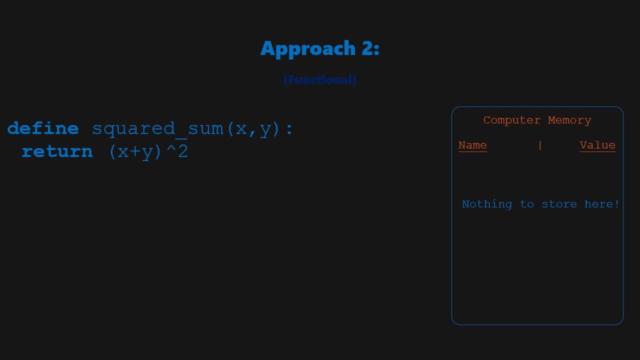 any side effects. No extra elements are created that would need to be managed by system memory outside of the function's scope, and no other state or object is changed outside of the function. With this approach, input is directly mapped to output. the parameters x and y are taken in. 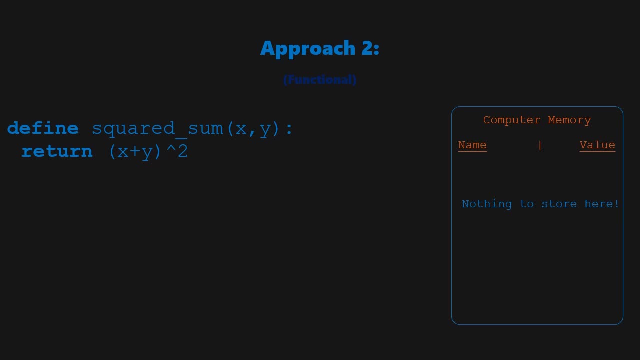 and their squaredSum is directly returned without any adverse effect or event taking place. In other words, this side effectless approach has a strict control flow, which is a critical part of functional programming. To recap, FP is a way in which a developer can solve a problem. This approach includes: 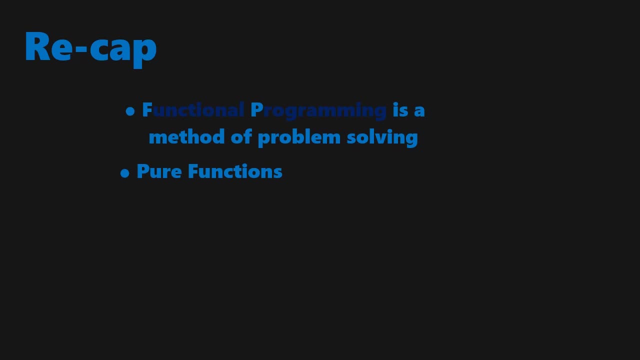 pure functions, meaning functions that don't include side effects, and a strict control flow, meaning directly mapping input to output. This style of programming is great for projects that don't tend to scale out, which would make them easier to maintain, test, debug and refactor. 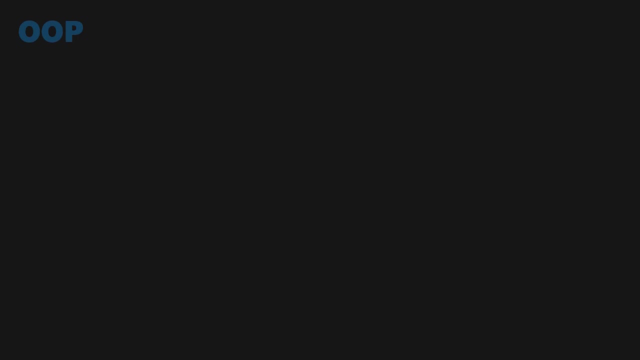 There are cases where object-oriented programming would be a better style to approach certain problems. Let's say I want to create a game involving a farm that has a bunch of animals. What would be a good way to go about programming them Well for each individual animal? 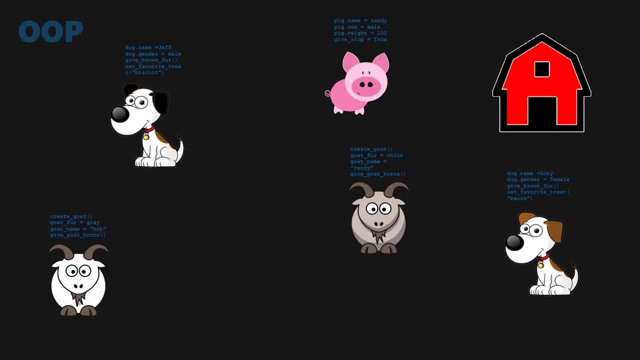 I could write specific code, over and over again, manually typing out all the redundancies between them and continuously repeating the process for every new animal I would like to add into the farm. This approach is not ideal. For every animal I have to start off from scratch and continuously. 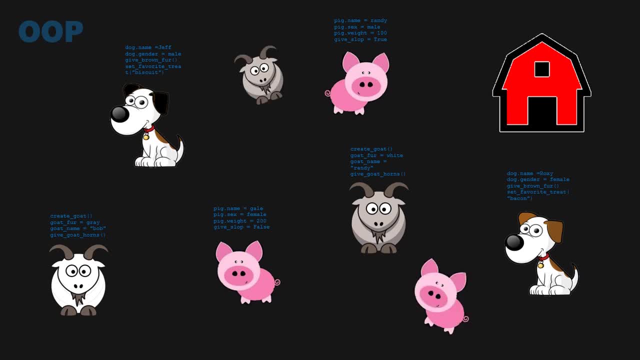 program every feature manually. If, for instance, I wanted to add 100 animals to my farm, this approach would take a vast amount of time and wouldn't be considered efficient. Additionally, after I have programmed all my animals, what if I discovered some bug in the 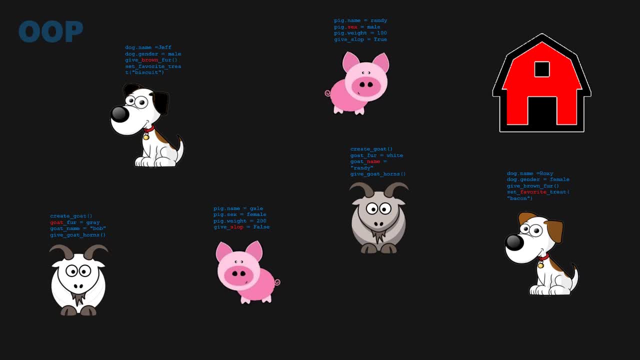 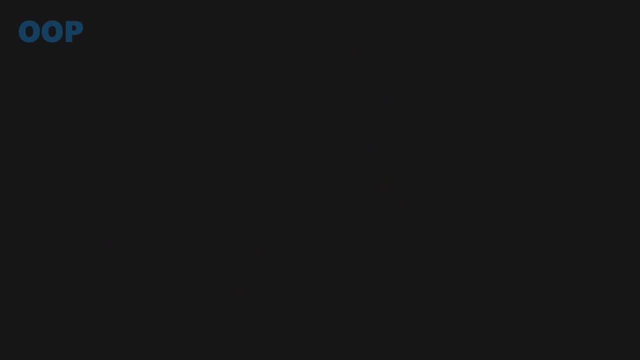 way I designed them. I would have to go back through each animal and rewrite their code, wasting even more time. What if, instead of individually programming each animal from scratch, I create a generalized blueprint of what an animal typically is and then apply that blueprint to every animal? I create Meaning? I only have to program. 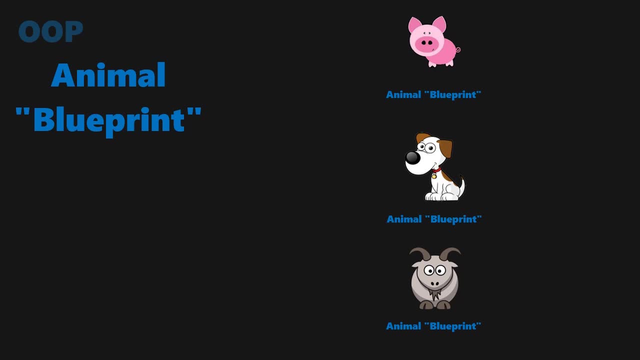 what an animal is once and apply that set of rules to each new animal automatically. This is a more object-oriented approach. The basic idea in this style of programming is the creation and use of these blueprints, which developers call classes. A class is like an. 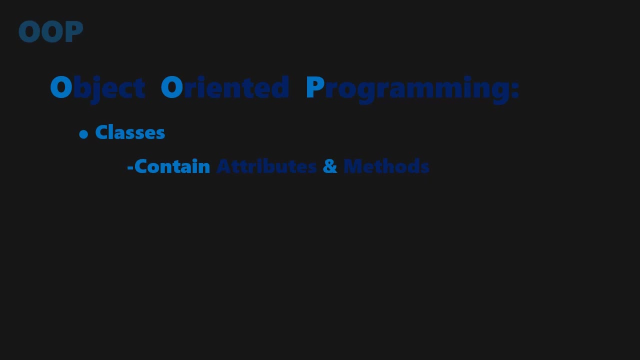 abstract blueprint that is used to describe some data with attributes and methods. Once a class is constructed, instances that inherit from these classes can be created, called objects. Each instance of a class can pass in data that the object stores and manipulates. according to the blueprint. 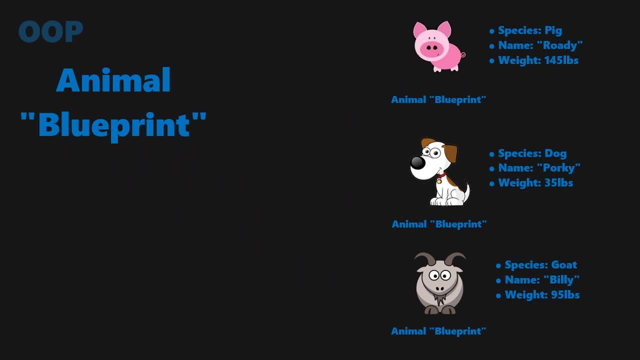 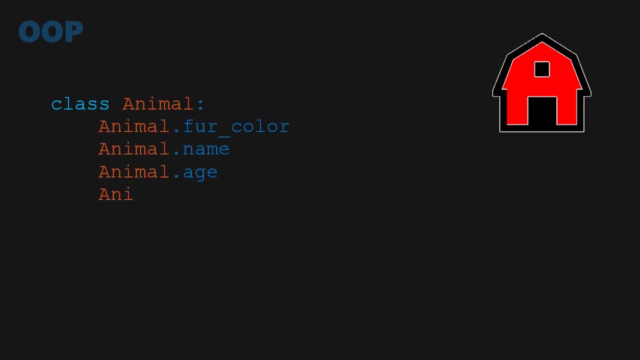 One can have multiple entities inheriting from the same class but holding different data. So, going back to the farm, I can create an animal class that can accept certain attributes, like fur name, age, sex, number of legs and so on. 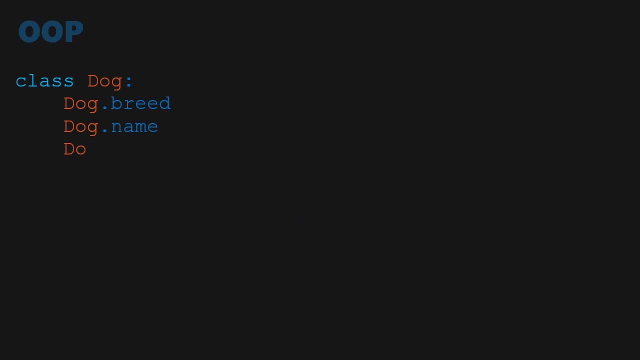 We can start off by making a dog class. This blueprint will accept the following parameters: breed name, age, sex and favorite treat. With this basic template, we can now create objects of dogs inheriting from our dog class by passing in values as parameters. 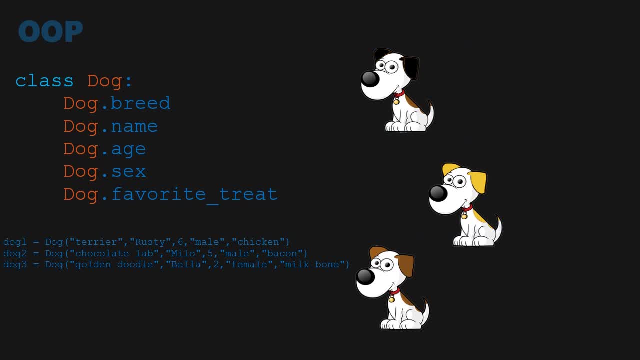 for the attributes of a dog. Each different instance of the dog class created here is held in the three variables dog1,, dog2, and dog3.. Dog1's name is Rusty and he's a terrier. Dog2's name is Milo and he really likes bacon.